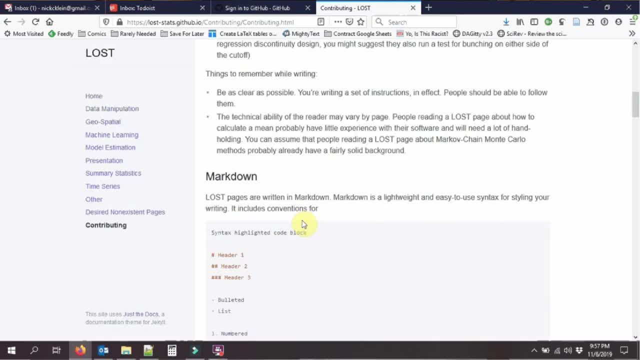 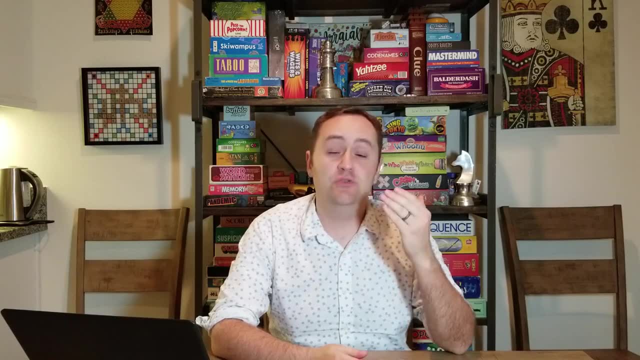 you in a lot more detail than this video is going to, all of the things that go into a LOST page and the specific technical details about how to edit a LOST page, including how to use Markdown. If you've never used Markdown before, don't worry, it's very simple. If you ever sent a text message. 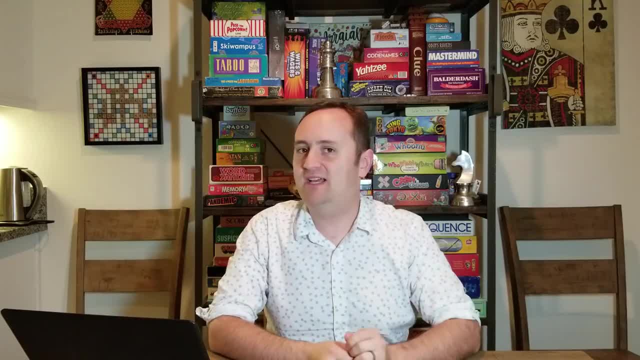 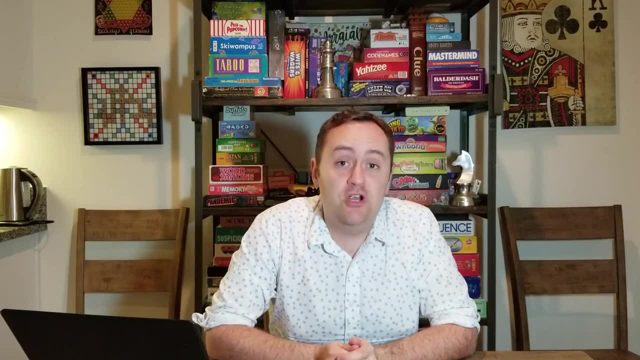 and used some asterisks to indicate bold, because you wanted to really emphasize something. that's about the level that Markdown is on in terms of difficulty, so don't worry about it. Once you've read the contributing page, then you're going to be able to contribute. 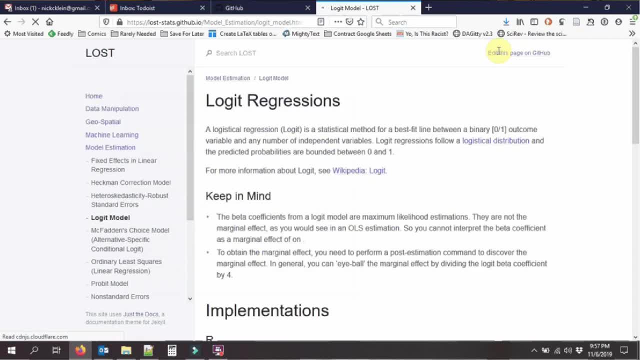 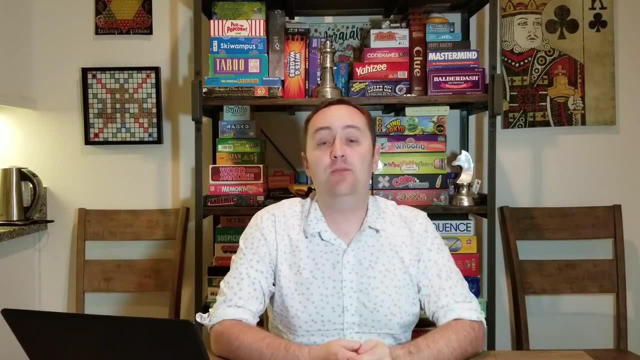 So all you have to do is to go to the page that you're interested in editing and find the edit this page on GitHub link up at the top right. That's one way. Or, if you're creating a new page, go to the GitHub repository and find the new page template that you can copy and start working on. 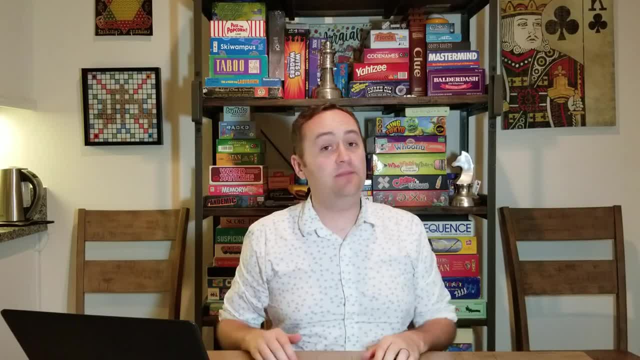 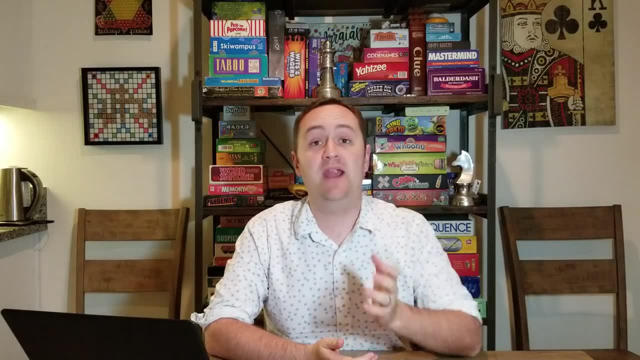 that. So now you've got the text that you are working on. Either you're editing something that already exists or you're creating a new page, writing through a template. There are four pieces to this page that you're going to want to think about, especially if you're writing a new page. 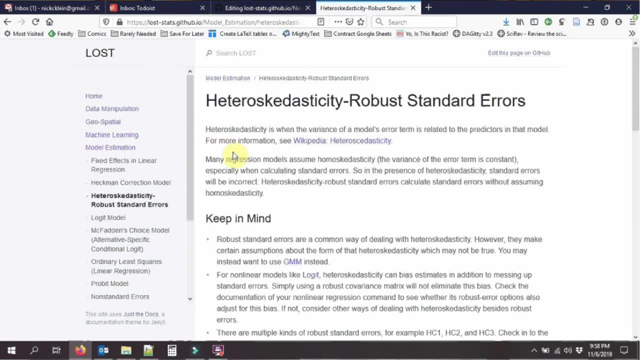 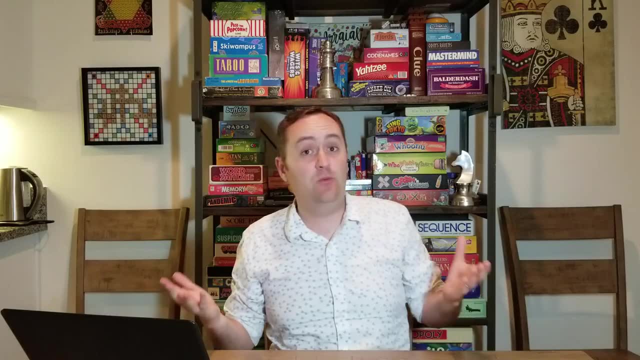 of your own. The first is the introduction. This is a very brief description. This is a very brief description of what that technique happens to be about. You don't have to go super far into detail. In fact, if you want, you can just do a couple of sentences saying what the technique is and 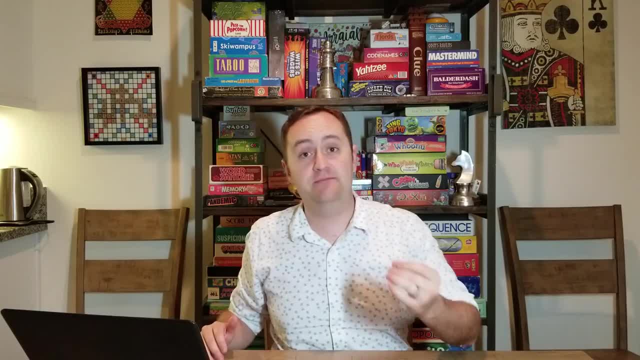 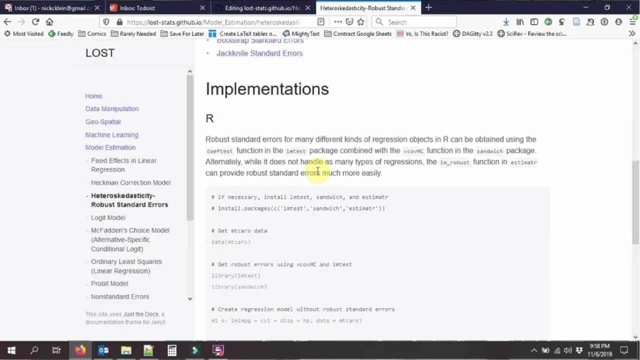 then link out to something like Wikipedia or some other resource that has more technical detail about the technique. The other three sections are going to tell people basically what to do. One of those sections is implementations. This is one of the key ones. This is going to describe how to. 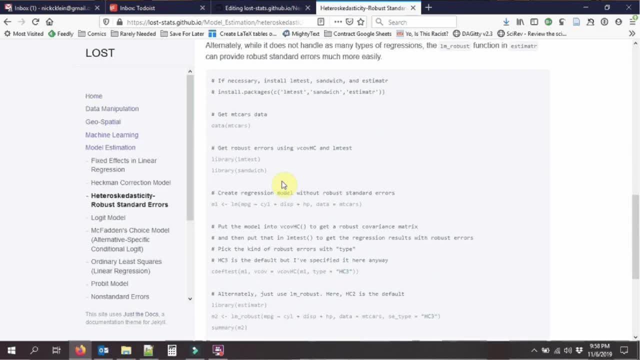 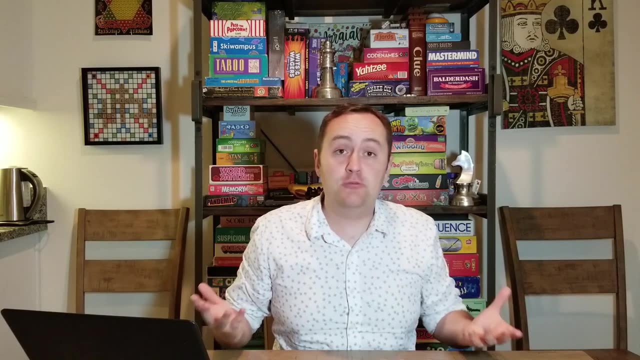 carry that technique out using an example that you will provide in the language of your choice or multiple languages perhaps. Maybe there's multiple ways to do something in a language. In that case, you know either pick the best one or present a couple of different options for the reader. The other two important parts are: 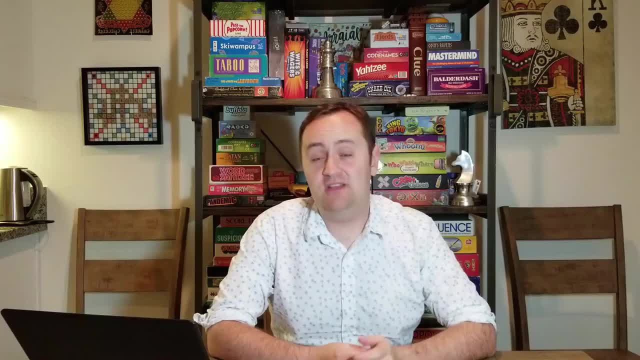 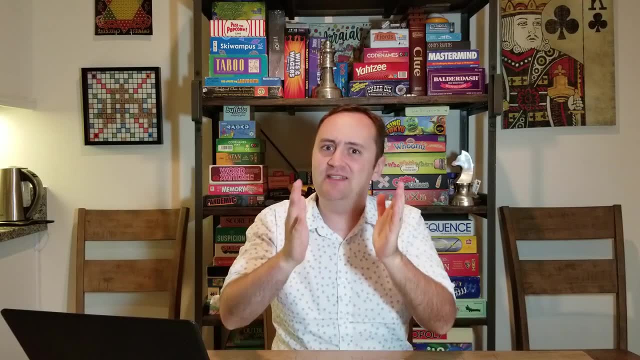 the keep in mind section and the also consider section. The keep in mind section is all about best practice and making sure that people know what they're doing when they carry out your technique. If you've ever seen somebody try to do a statistics technique and do it all wrong. 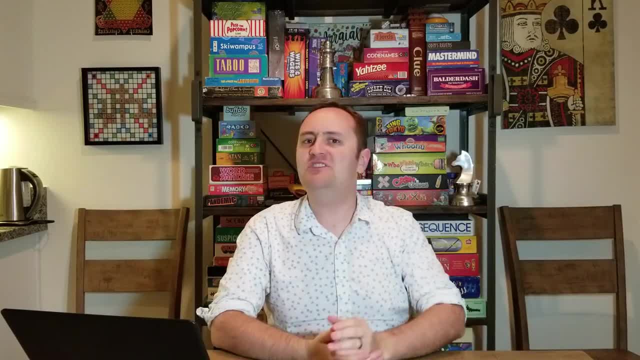 well, here's your chance to try to catch that before it happens. So any assumptions that people should be aware of when they're using this technique, or perhaps knowing that they have to do something that they're not familiar with, they're not familiar with, they're not familiar with the 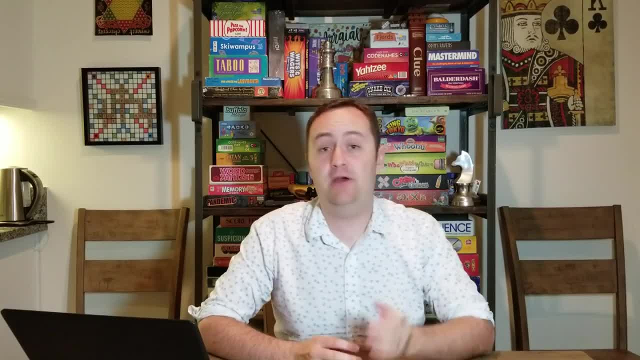 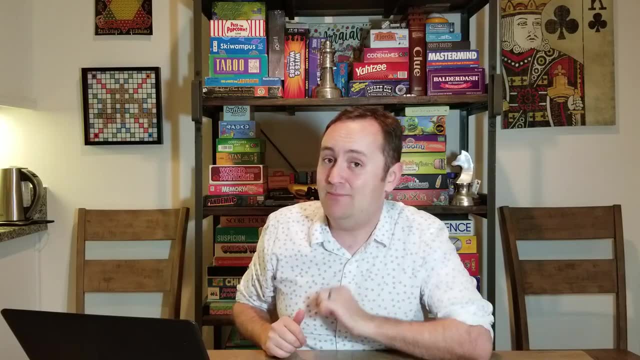 data before they do it. For example, let's say you're writing a page about lasso regression. Now when you're doing a lasso regression, you should really standardize your data before you do it. That should probably go in the keep in mind section. The other section is the also consider. 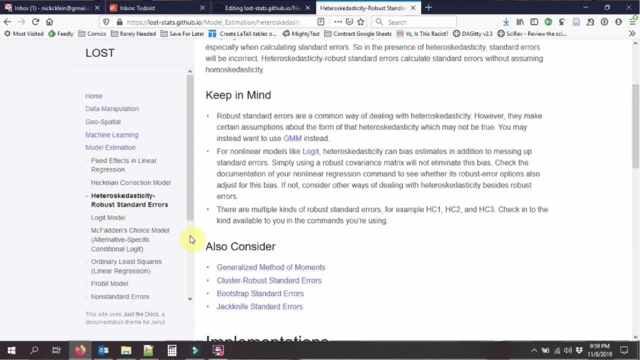 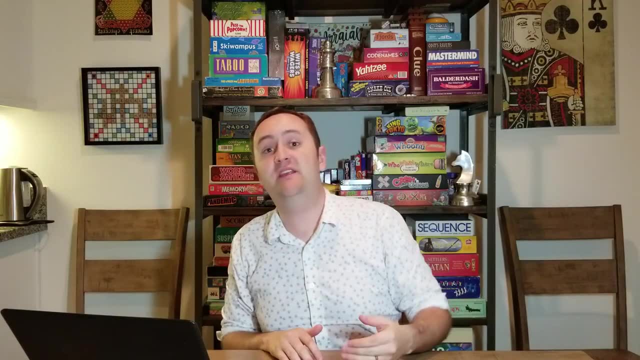 section. This is going to be other techniques that you might want to carry out in addition to the one that you are currently doing, or perhaps instead of the one that you're currently doing. So, for example, if you're running a regression, you might want to consider different kinds of. 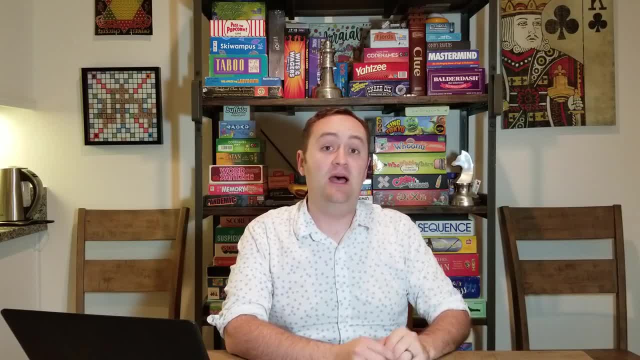 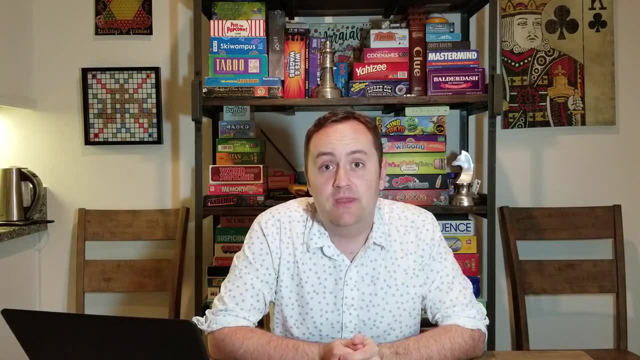 adjustments you could make to the standard errors of your regression, And so you might link in the also consider section to other lasso pages that would describe certain ways of adjusting your standard errors. So that's pretty much it. So you've got your page. You've edited in what you. 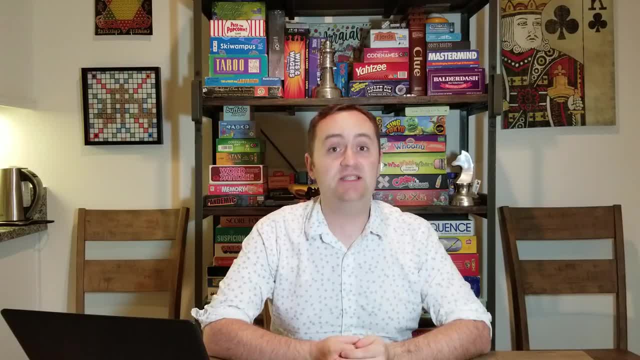 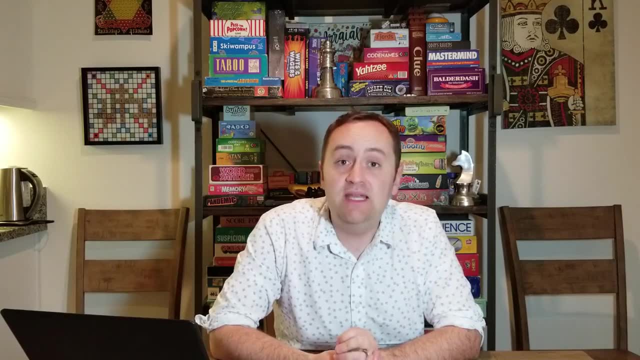 want to do on the page, or you've created a brand new page from the template that exists. Now, how do you actually get your work on lasso? Well, there are two ways to do it. If you do happen to know how to use Git and GitHub, you can fork the repository, make your changes there and then do. 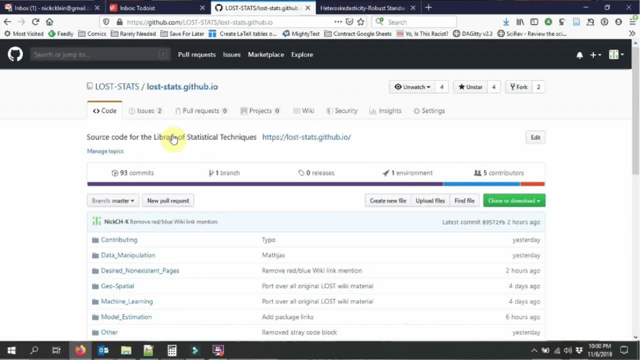 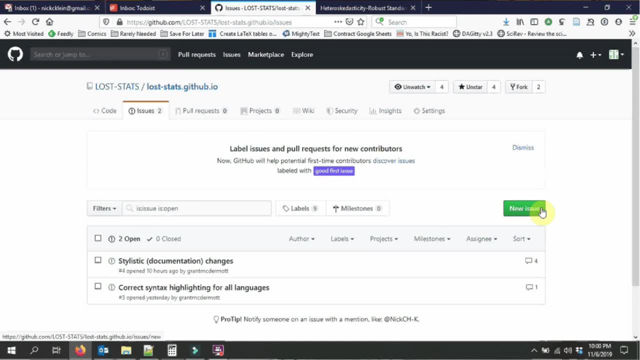 a pull request to have your changes brought back into the main repository. If you don't know how to use GitHub, that's totally fine. You can go to the issues page, which you can find in the GitHub repository, and you can post a new issue asking to be added as a contributor Once you are. 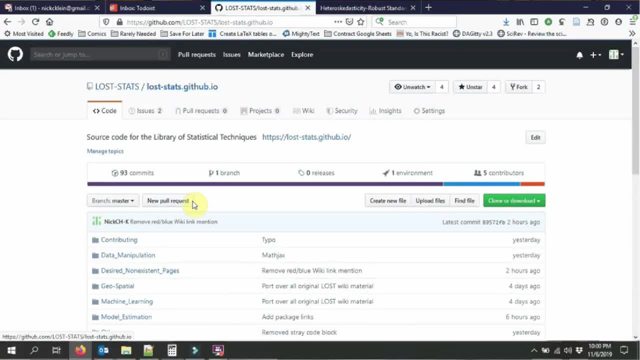 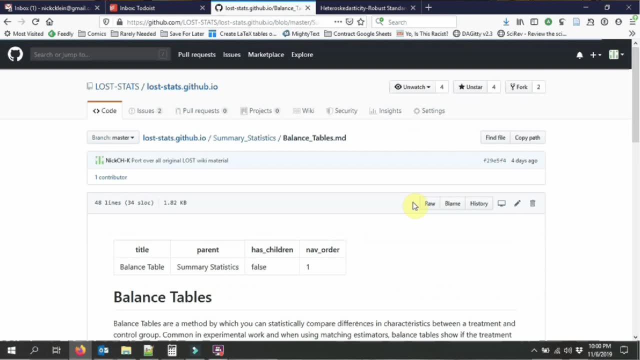 made into a contributor. you can simply directly edit the text files that are in the GitHub repository and make your changes. that way, We will also make you a contributor after you have successfully submitted a pull request. So either way, you should end up as a contributor, which is 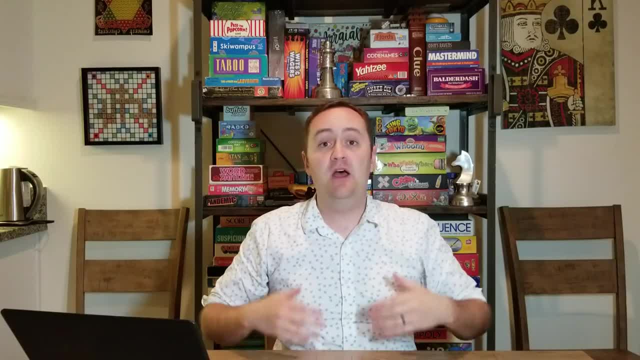 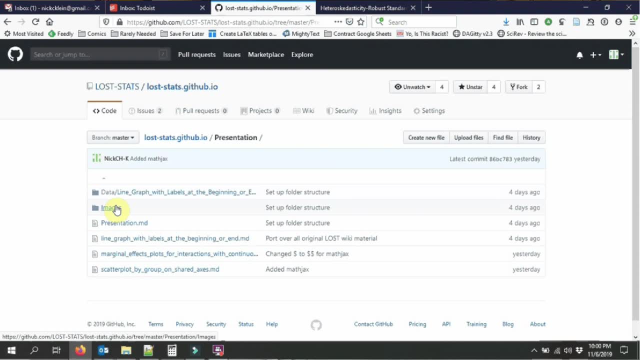 just fine, And there's lots of things you can do here. We're pretty flexible on the different kinds of ways that you can contribute. You can add in your own images. You can upload images to the images subfolders of whatever category you're looking at. You can also upload data. You could. 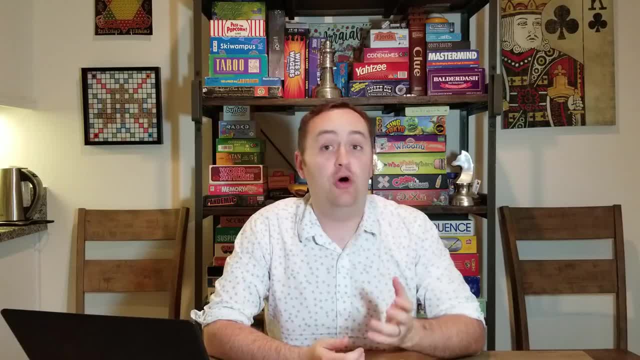 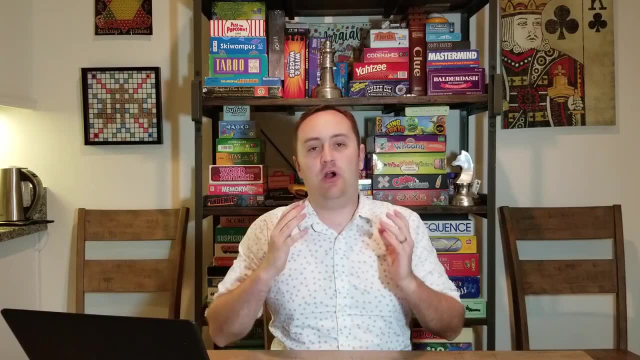 upload a shared data file that can be used in all of the examples in all the different languages on a page, and then each of those individual examples can load that data file directly. All of these details are on the contributing page as to how to do these specific things. 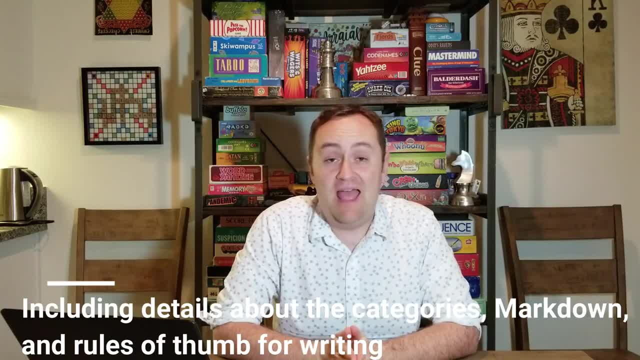 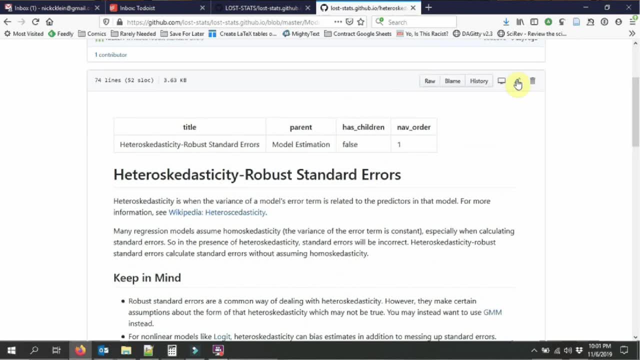 but you might as well just get started. Find a page that you think could have a little edit on it, click the edit this page on GitHub button and add in the information that you have. You can get started. We're very interested to see what you.